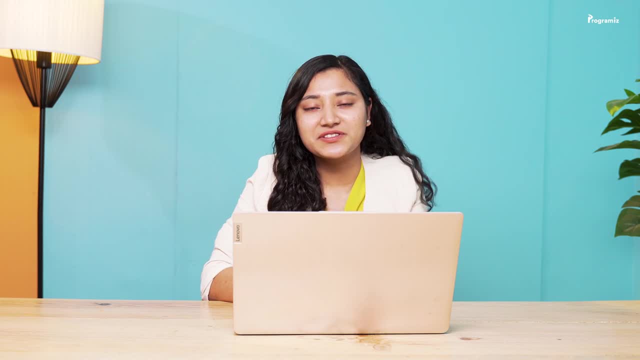 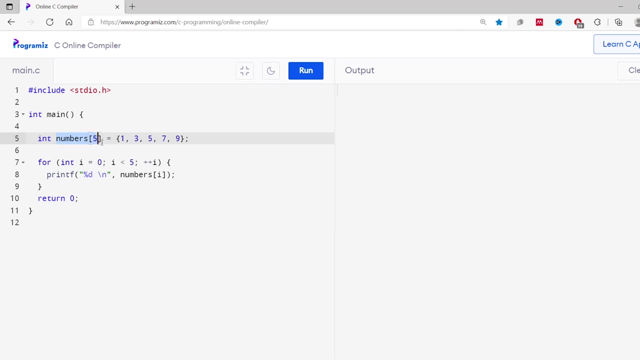 Now let's try to access these elements using pointers, But first let's try to access the memory address where these array elements are stored. So here we have our array of numbers and we are printing The array elements using printf statement inside the for loop. 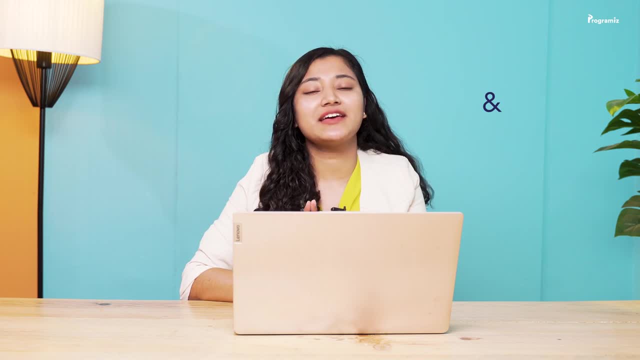 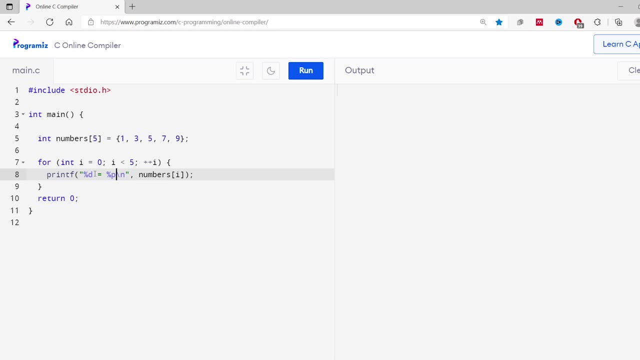 Now let's print the address of each element using the ampersand operator. Let's modify this print statement. I'll add here percent p and here comma ampersand numbers. bracket i: I have used percent- p format specifier to print the memory address. 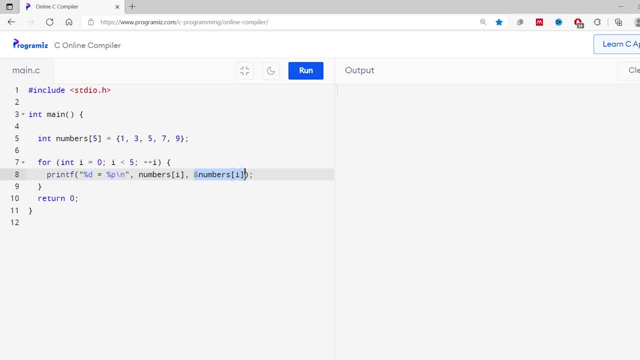 And here I have used percent p format specifier to print the memory address. And also I have used here ampersand number square bracket i to print the memory address of the i-th element. Now let me run this code. As you can see, we get the corresponding address of each element. 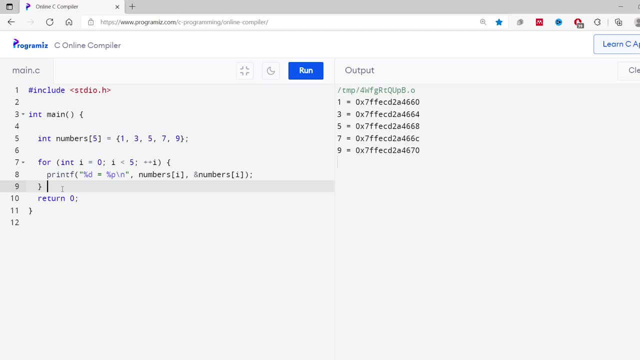 Now let's see something interesting. For that I'll print the address of array without any array index. So I'll use printf statement printf here. array address, percent, p, comma numbers. Now let me run this code Here. if you look into the output you will notice two things. 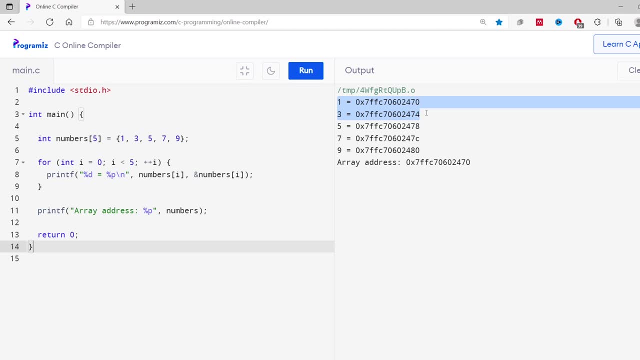 First, the difference between two memory addresses is 4.. This is because the array is of integer type and size is of int is 4 byte. Second, the memory address of the for loop, The first array element and the address of the array, is the same. 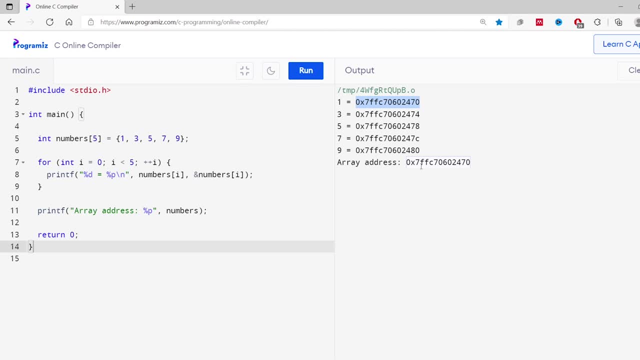 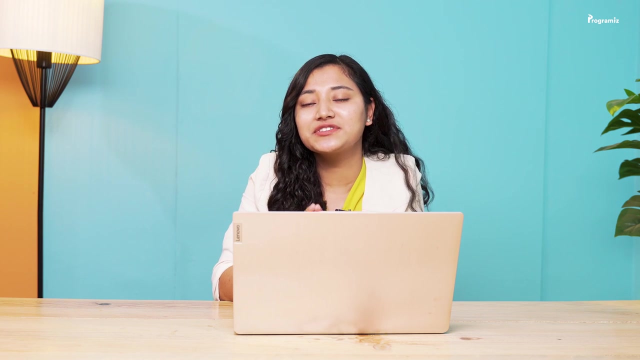 This is because the address of array always points to the first element of the array. Also, here we have used only the name of the array, without the ampersand sign. This is because in most context array names are by default converted to pointers and we can directly use the name of the array. 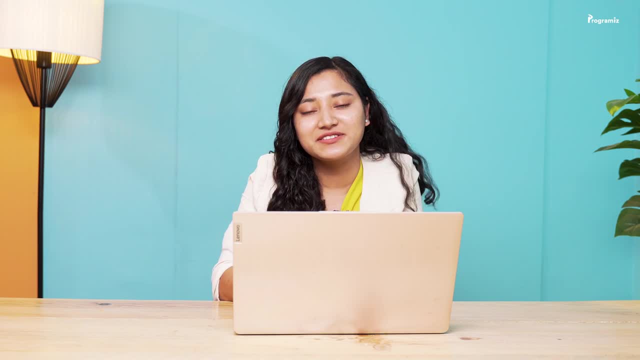 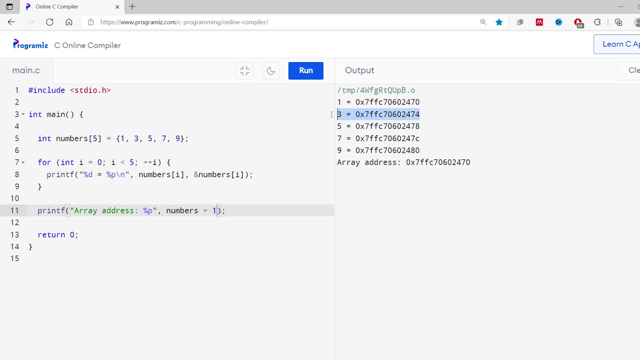 So from now on, if I use array name, remember it's the pointer. Similarly, we can use number bracket. We can use number plus 1 to print the address of the second array element and we can use number plus 2 to print the address of third array element. 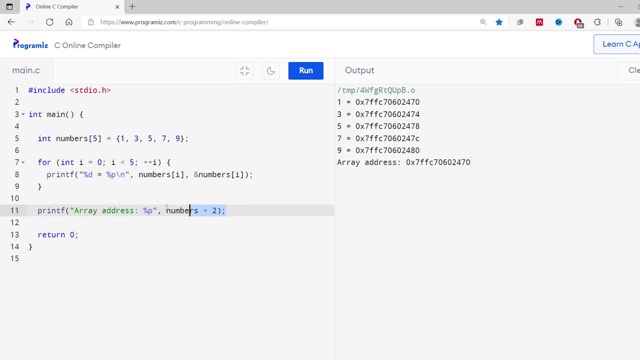 Now let me show you that. So what I'll do is I'll copy this and I'll paste it here and I'll modify this print statement to have a clear output. So array address of 1, backspace n, And I'll change this to numbers. 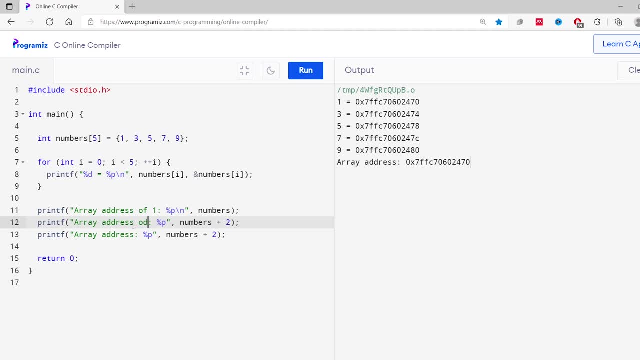 Then array address of 3.. Here I'll add here backspace n and I'll change this to numbers plus 1 and I'll change this to array address of 5, and let's put this as it is. Now let me run this program. 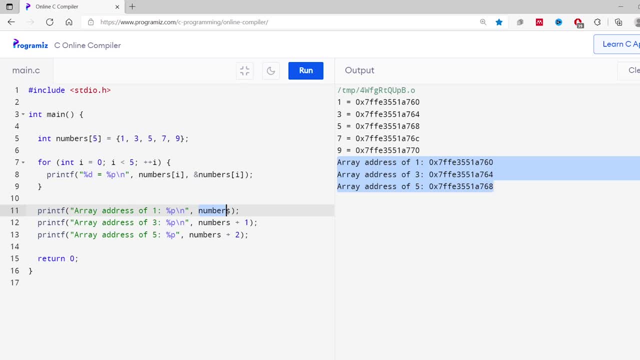 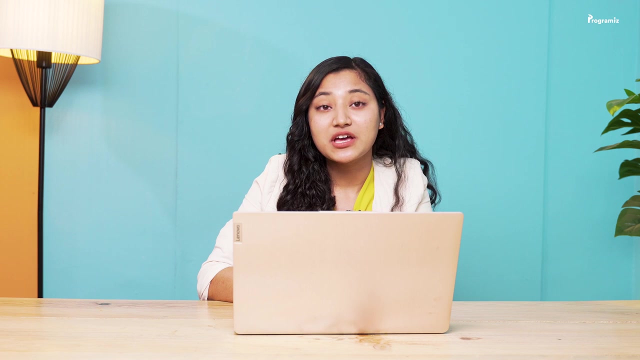 As you can see, this number gives the address of first element, and numbers plus 1 gives the address of second element, and numbers plus 2 gives the address of third element. In this way, numbers plus i gives the address of ith element. So we can implement this exact logic in a loop. 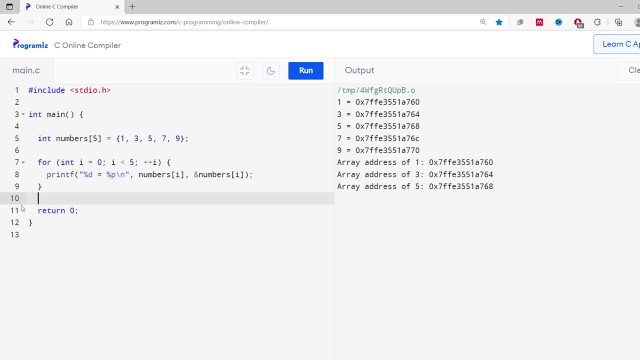 So I'll modify this code. First I'll remove this print statement And in this print statement I'll modify this. So I'll use ampersand numbers, bracket i to number plus i. So number plus i. Now let me run this code. 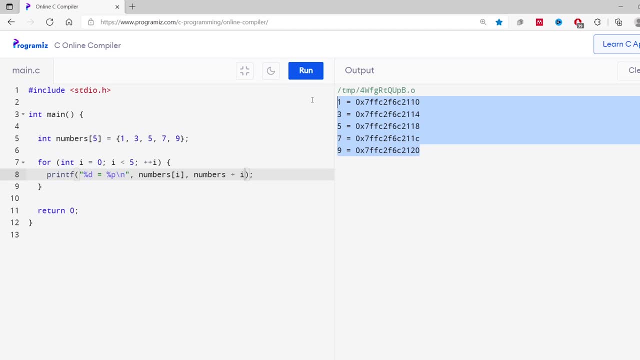 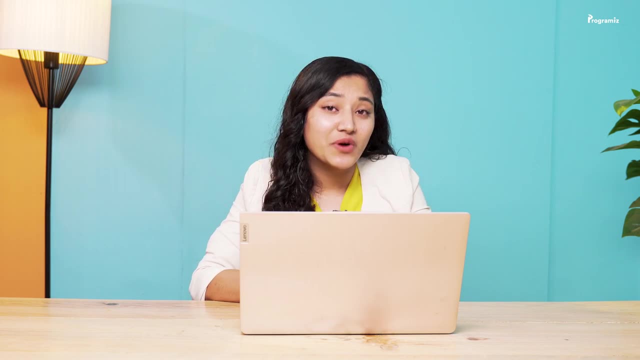 As you can see, we get the desired output. By the way, do you want to take your programming journey to the next level? Watching tutorials is fine, But it has one limitation: It is hard to learn and practice together at the same time. 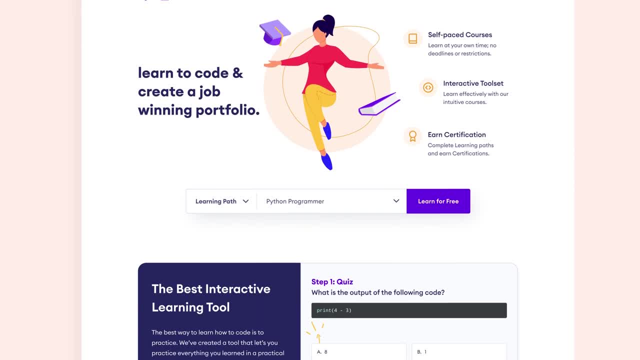 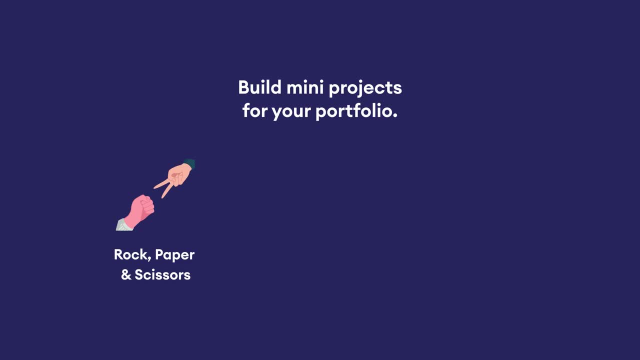 Lucky for you, We have recently launched ProgramEase Pro that provides tutorials along with quizzes and challenges, which will help you practice and test your learning in real time. Also, the course includes projects to give you an experience of how programming works in real world. 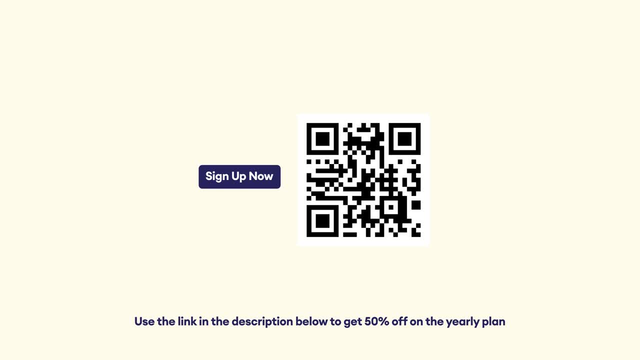 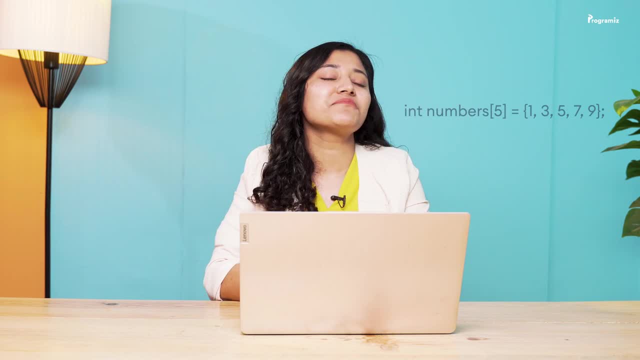 Sign up now. Visit this link, which is also available in the video description below. In our last example we saw that for an array numbers, numbers is a pointer that gives the array of the first element. Similarly, numbers plus i gives the address of first element. 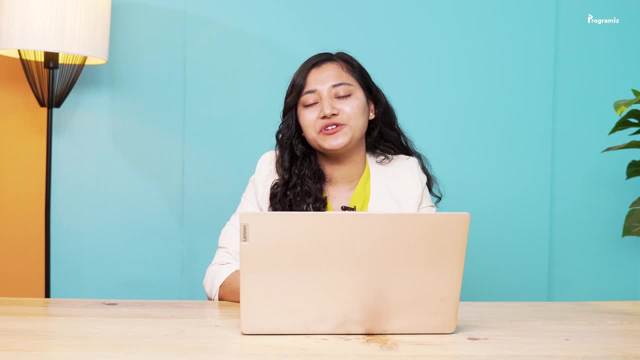 Number plus i gives the address of the ith element. Now we can use this pointer to access the array elements. To access the first element, we can use asterisk number. Similarly, to access the ith element, we can use asterisk parenthesis numbers plus i. 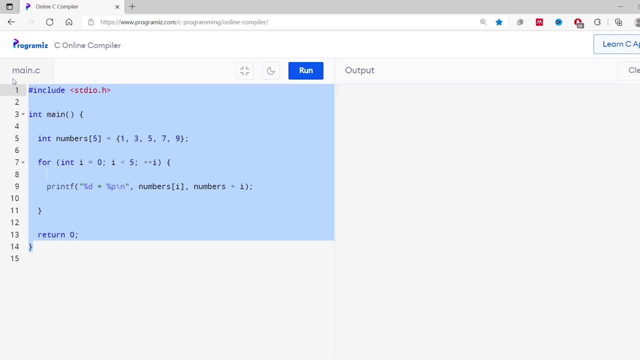 Let me show you. You can see the code from our earlier program Here. numbers plus i gives the address of the ith element. Since I want to use the pointer to access the element, I'll remove this number bracket i from here. Instead I'll write asterisk parenthesis. numbers plus i. 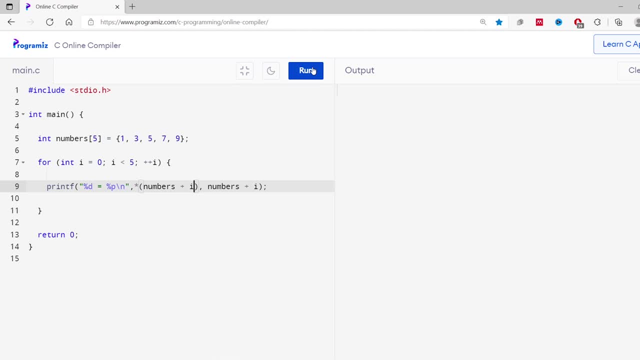 So this gives us the ith element. Now let me run this code As you can see: number plus- i gives the address of the ith element And asterisk parenthesis, number plus i gives the value present at that number plus i address. 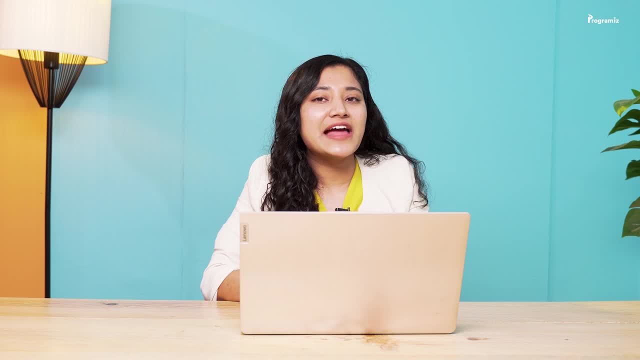 In this way, we are able to access the address and value of an array using pointers. Okay, guys, We need your support to keep these types of content free for all users. YouTube really likes engagement on the video, So leave a comment below. 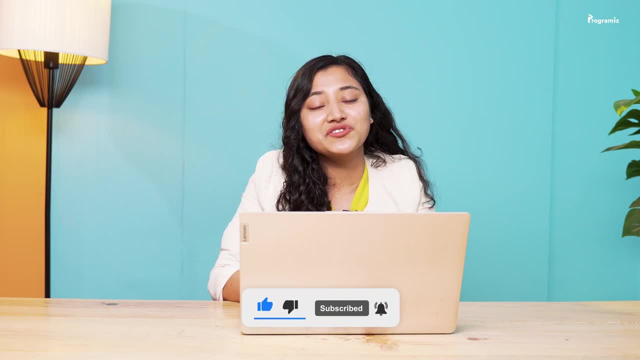 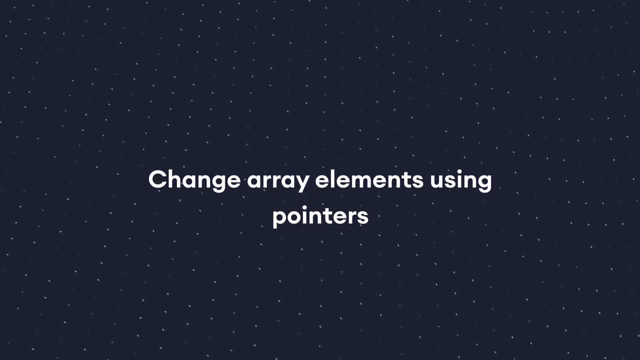 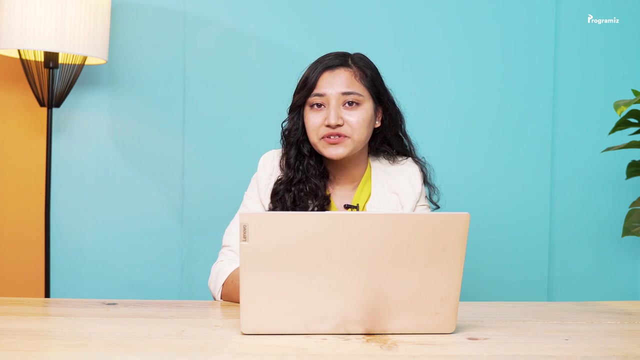 Press that like button, Hit subscribe if you haven't already. Let's get the engagement score high up so that more people can discover and enjoy these courses. Just like accessing the array elements, we can also change array elements using pointers. All we have to do is: 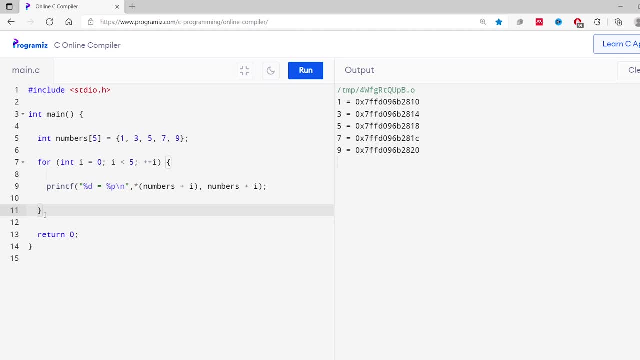 assign a new value to the address. Let me show you Here. I have the code from our earlier program. I'll remove this for loop. Now suppose I want to change the value of first element to 2.. So I can simply write here: asterisk numbers is equals to 2.. 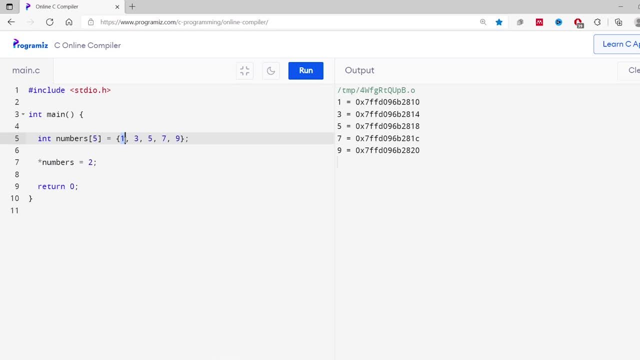 Here asterisk number represent the first element and I have assigned a new value to it. Also, let's change the last value to 11 from 9, so that our array includes only prime number. So I'll write here asterisk parenthesis numbers plus here: 0,, 1,, 2,, 3,, 4.. 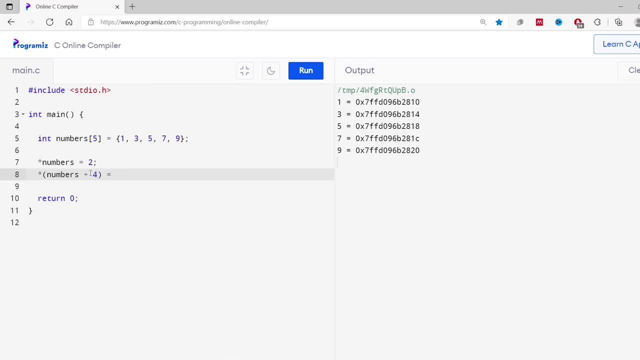 So numbers plus 4 is equals to 11.. Here asterisk parenthesis. numbers plus 4 represents the last element and I have assigned a new value to this address. Now to verify the value I changed or not, let me print the first and last value. 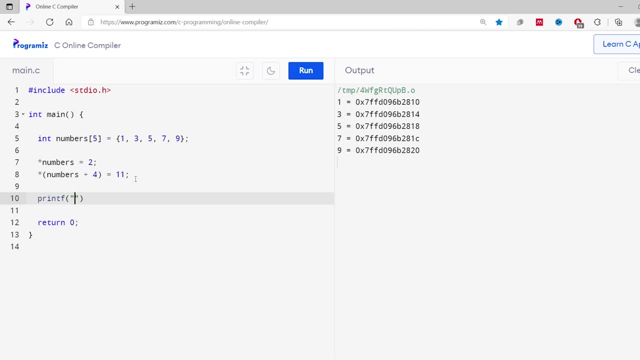 So I'll use print statement Here. first element is percent d, backspace n, comma, asterisk number. And another print statement Here. it prints the last element Here. last element Here, column percent, d comma asterisk parenthesis, numbers plus 4.. 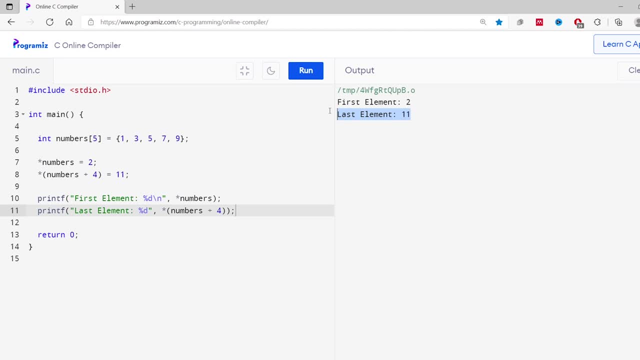 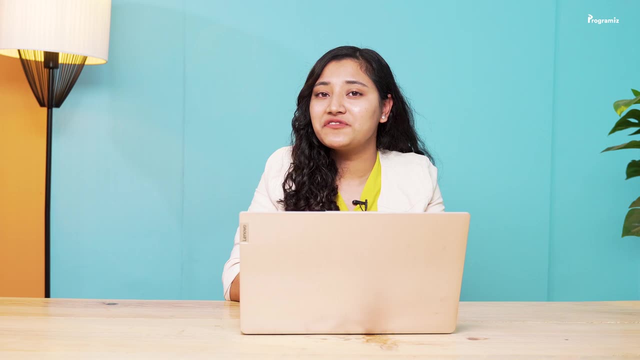 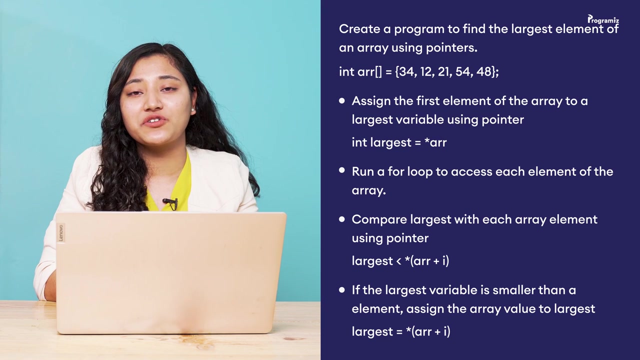 Now let me run this code. As you can see, the value of first and last elements are changed. Now to revise what you have learned in this program, here is a programming task for you: Create a program to find the largest element of an array. 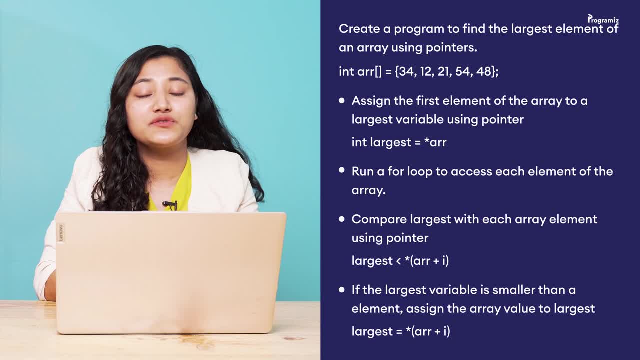 First create an array with elements 34,, 12,, 21,, 54, and 48. Then assign the first element to the array, to a largest variable. This time you should use a pointer instead. Run a loop to iterate through each array element. 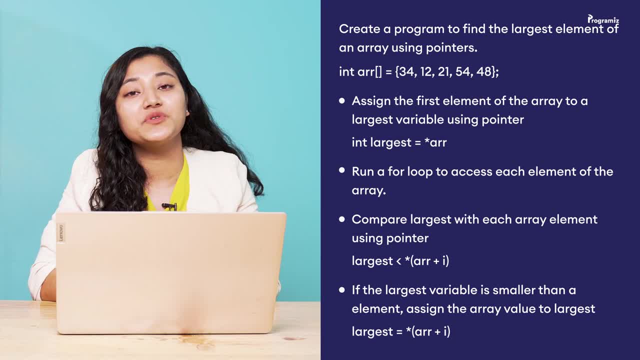 In each iteration of the loop, compare the largest variable with each element of the array using a pointer, And if the largest element is smaller than the array element, assign the array element to the largest variable, Again using pointers. Finally, print the largest variable. 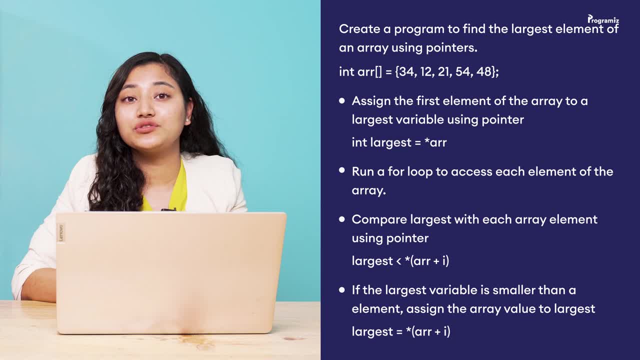 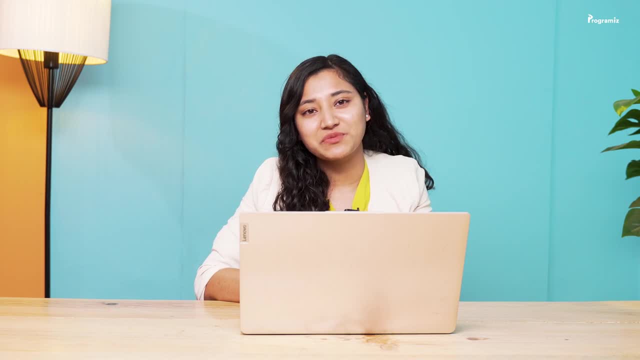 You'll find the answer to this question in our Github repository And also, if you want to revise this concept, all these programs will be there as well. I'll put the link in the video description below, Now that we have reached the end of this video. 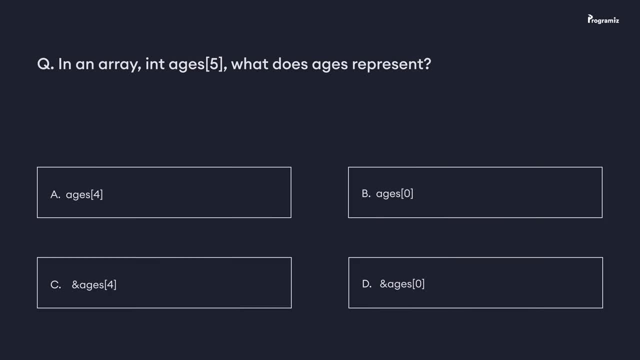 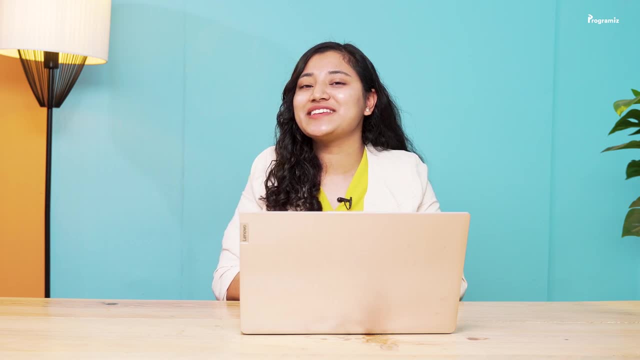 it's time for programming quiz In an array int, ajs. what does ajs represent? Comment your answer below. See you in the next video. Happy programming, Thank you.